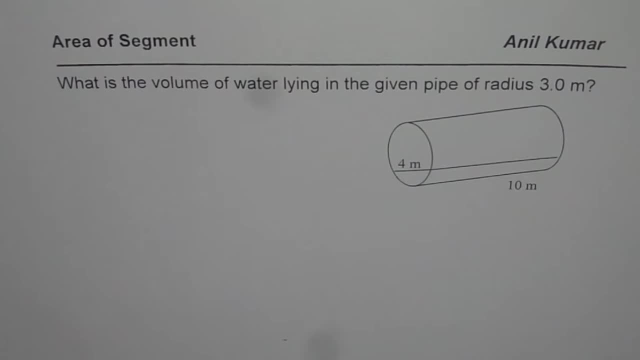 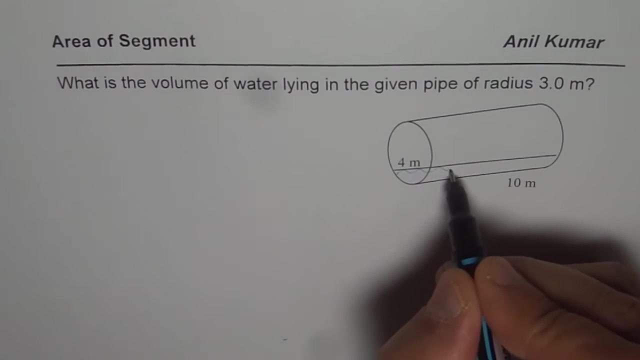 I'm Anil Kumar and here is an excellent question on application of the area of segments which you have learned so far. The question here is: what is the volume of water lying in the given pipe of radius 3 meters, right? So that is the water for us. So we need to find the 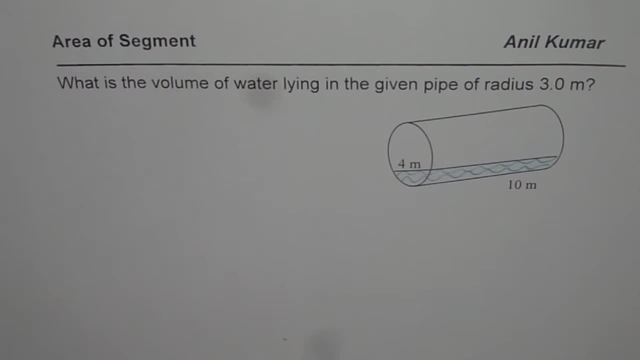 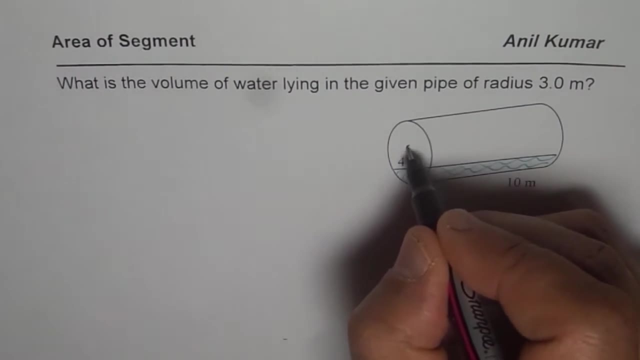 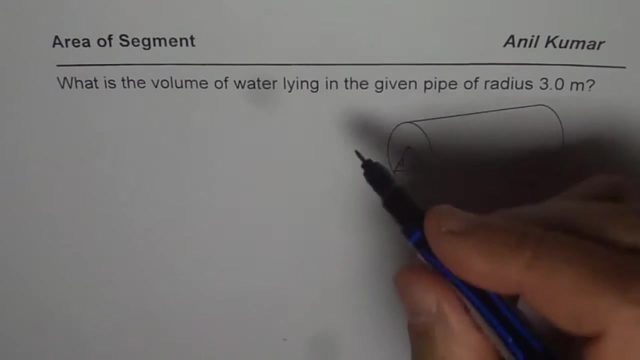 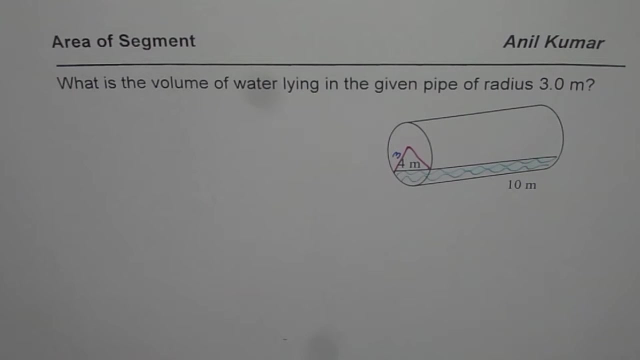 volume of this water. What we are given in this particular case is that the pipe has a radius of 3.. So if this is my center, then joining this center will be kind of a triangle whose radius is 3.. So this is what is given to us. We need to find volume of the water. 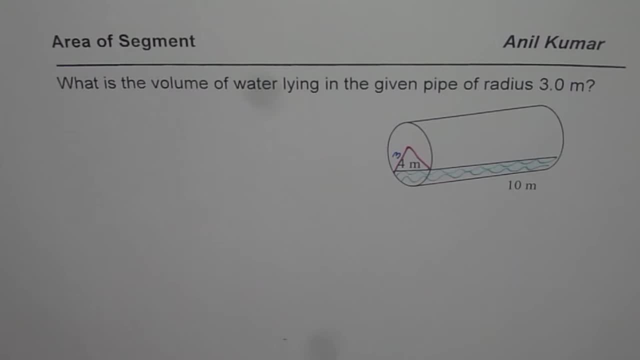 So to find the volume of the water, what we can do is we can find area first of the water- in this this is called segment- and then multiply with the length of 10 meters to get the volume Correct. So first step for us, basically, is that we need to find- let me make a big circle- 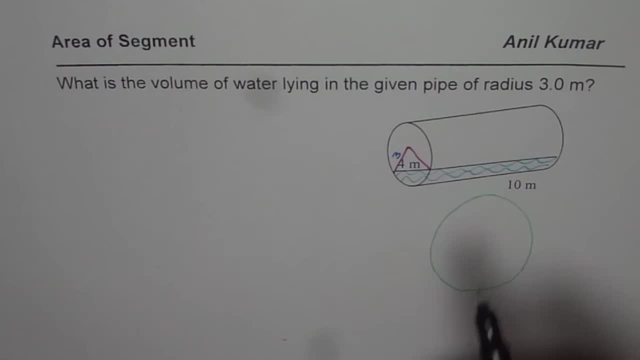 here. Well, it's not all that good, but still I think it can work for us. Let us say: this is a small, this is our chord in this particular circle. Let's say that is the center, Okay, So I'm trying to make it slightly bigger so that you know it helps to write down all. 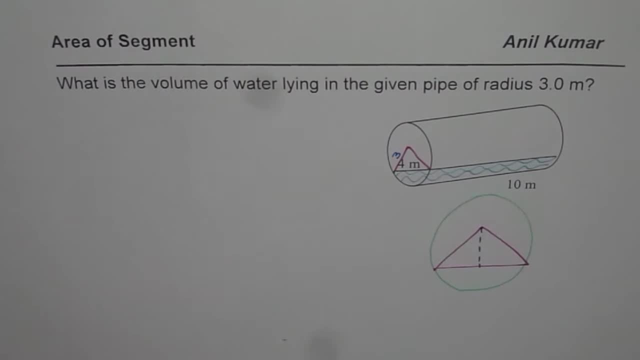 values and calculate. So in this particular situation, what we will do here is we'll find area of the segment. So this, this portion here, is called the segment, So we'll find the area of this which is segment. Once you find area of the segment, we can multiply by the length to get the volume. 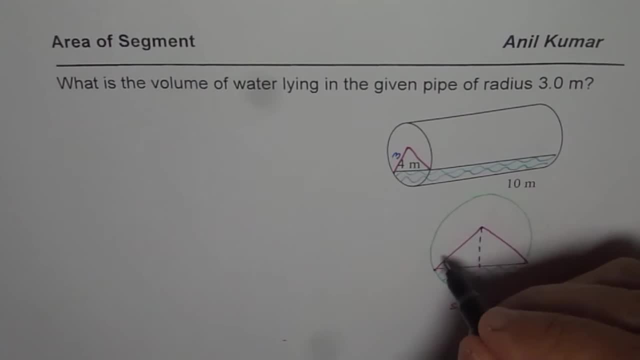 I hope you get the concept, So at this stage you can actually pause the video and answer the question. So what we have here is a triangle whose sides are three centimeter. Now that's an isosceles triangle. radius is same, So it is going to divide this chord into two equal 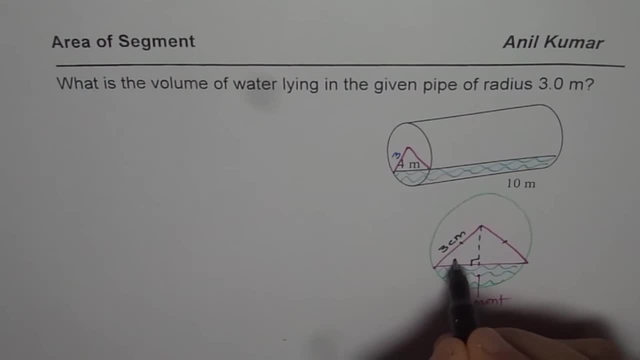 parts, Since four is the total length. each will be two right. And let us say: this angle for us is we need to find this angle correct. So let's say this angle is theta for us. Okay, Let's find the angle first. 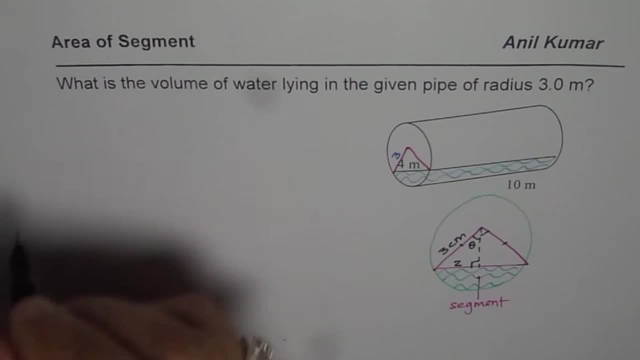 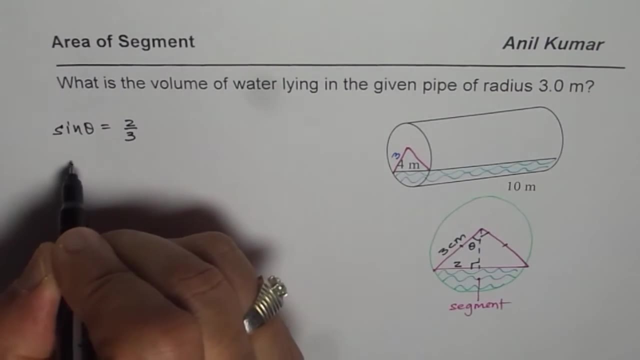 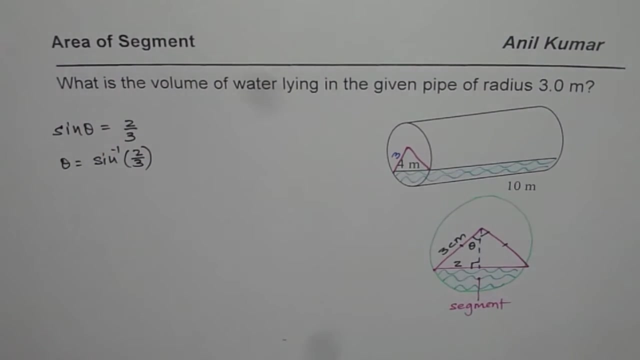 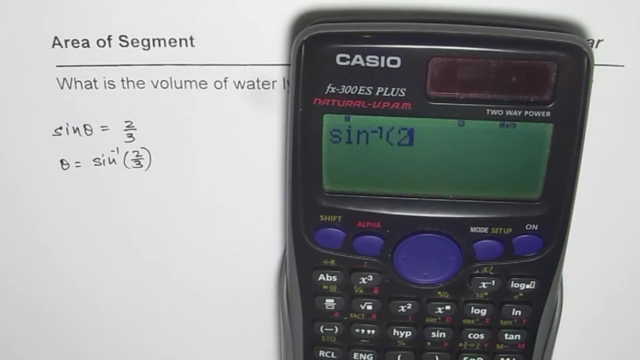 So we know from this triangle. let's solve for the angle. So we say: sine theta is equals to two over three. So sine theta is two over three, that means theta equals to sine inverse of two over three. So let's find how much theta is. So we have sine inverse within brackets: two divided. 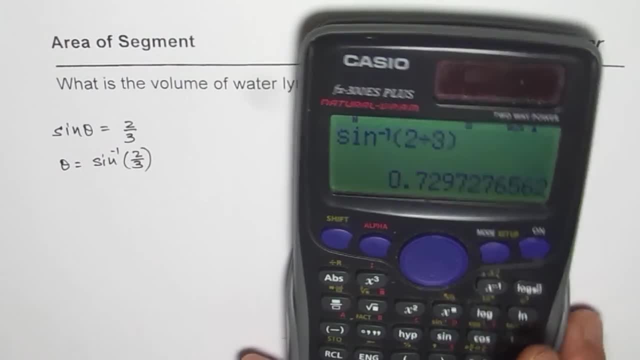 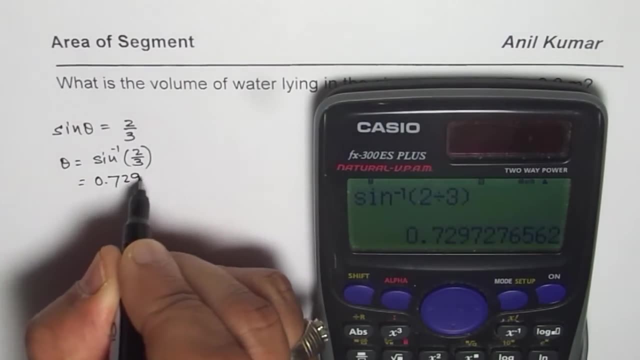 by three equals to 0.729.. Cool, Cool, Thank you. All right, So that's the angle. All right, That's the angle. All right. That's the angle. 9, let me write down here- is equals to 0.7297. it's good to take four decimal places, it is all in. 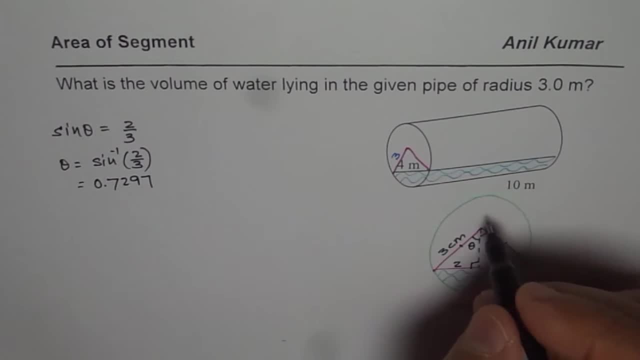 radius. okay, so we found the angle. so this is, let us say, center o. let me call this point a and b and let me call this midpoint as as m. okay, so in that case, what is om? we need to find the height. we know the base of the triangle, correct, which is four, two plus two. so om we can find. now we know. 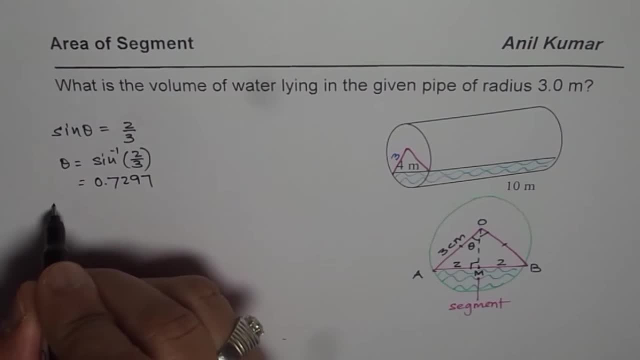 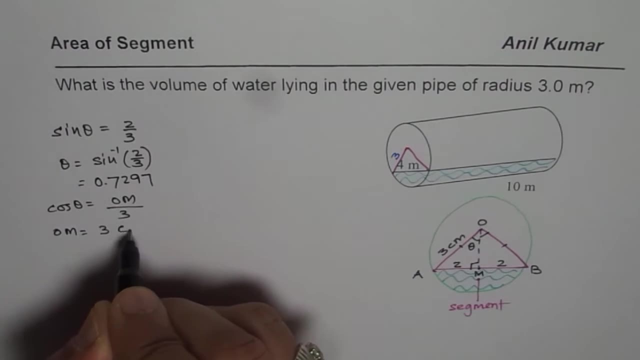 the angle using cosine, correct? so we have cos. theta equals to om over three, or om equals to three times cos of this angle, which is 0.7297, right? so let's calculate om. so we already have the angle. we'll say cos of the answer. 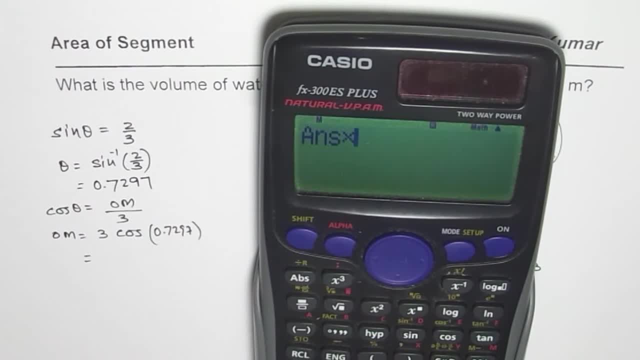 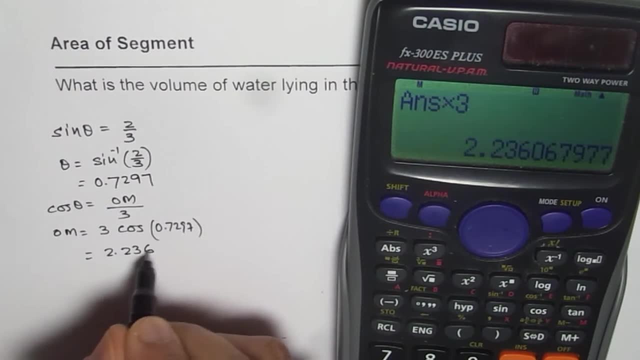 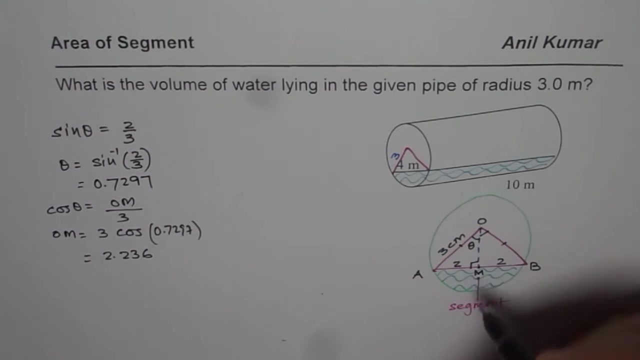 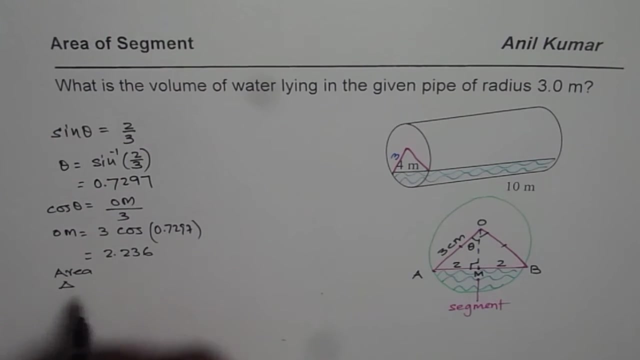 and we'll multiply that by three so we get two point two, three, six. so this is two point two, three, six. okay, two point two, three, six. so that is om for us. okay, so that gives us the area of triangle. so now we can say: area of triangle, which is aob is equals to half of base ab. 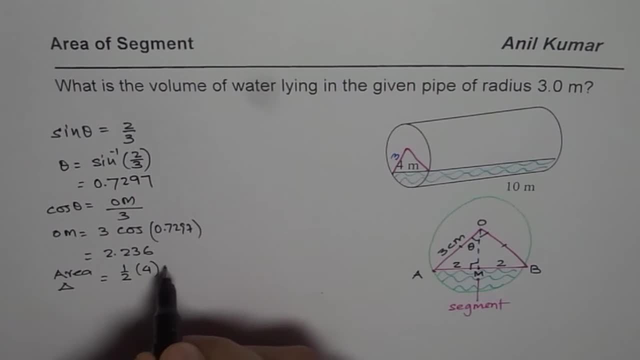 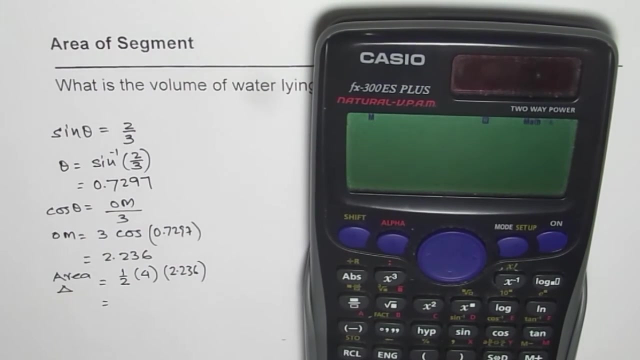 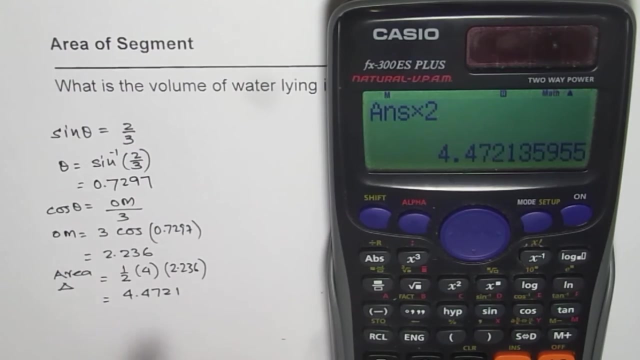 ab is four for us right b times height, which is om two point two, three, six, correct. so let's calculate this value. we already have two point two, three, six. well, multiply by two right four point four, seven, four, seven, two, one. okay, so that gives us the area of the triangle. well, these were. 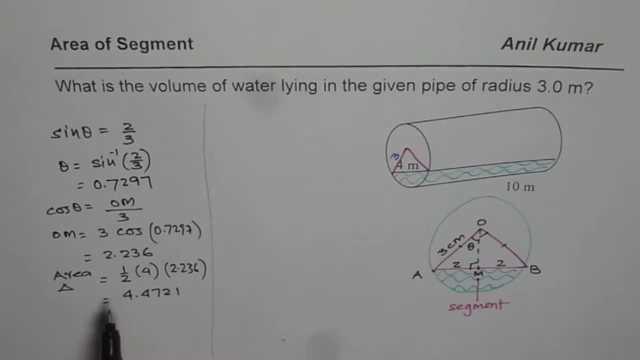 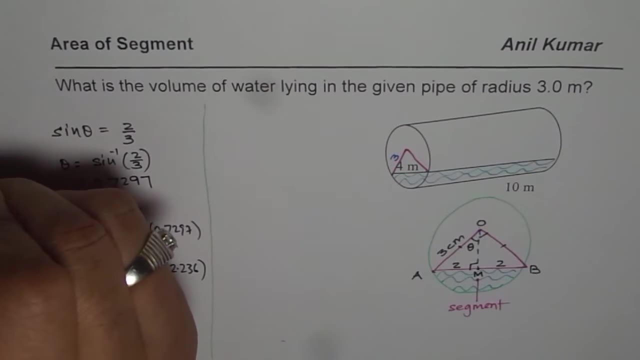 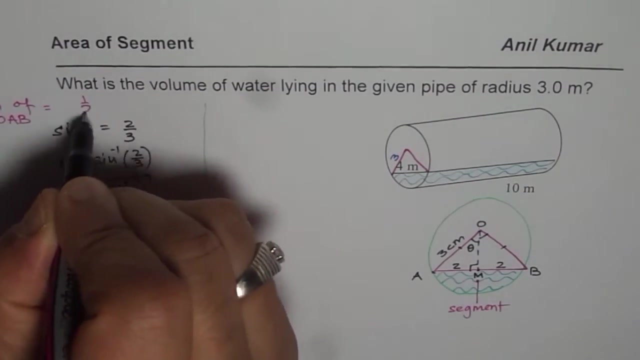 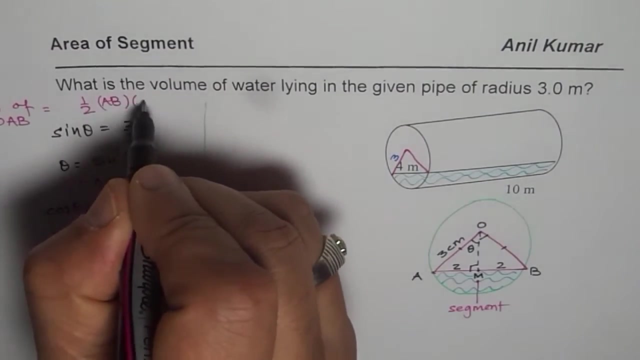 many calculations at one place. i hope you understand what we did right. so first step was to find area of triangle. so it is. what are we trying to find? area of triangle, oab side, which is half base, which is ab times om the altitude right, so ab times om. now we did all this to find what is. 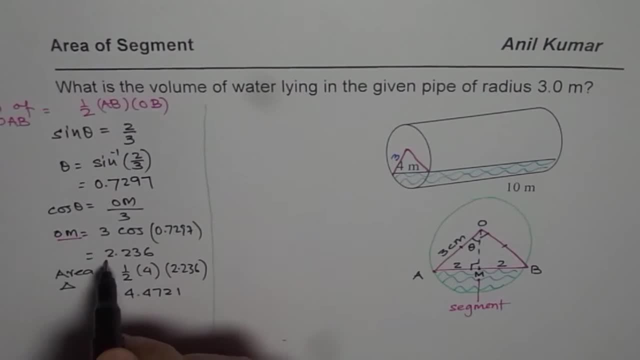 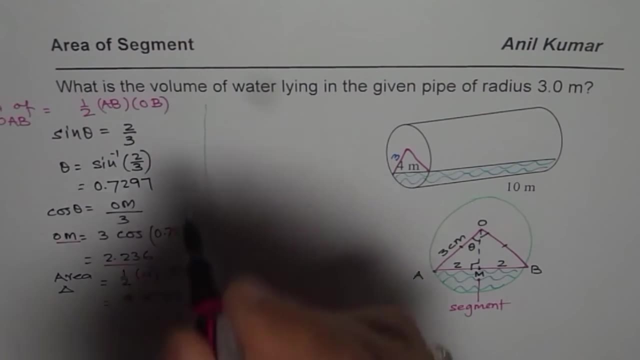 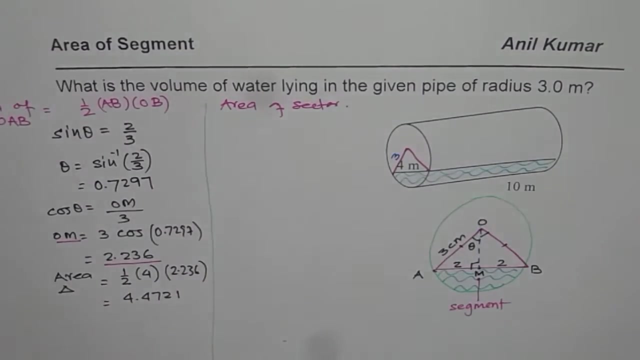 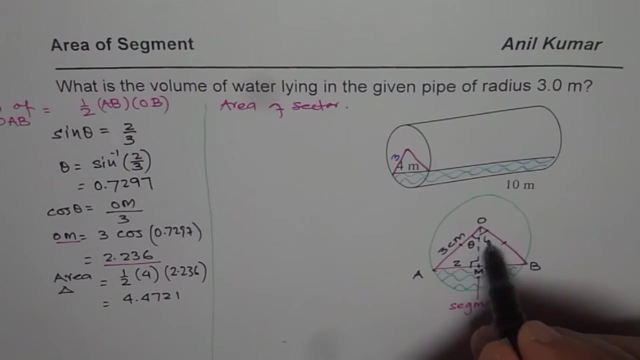 om, right? so we have to find what om is. and that was found to be this much using cos, right? so this is the calculation we did. now let us find area of sector. okay, now to find the area of sector. it is the ratio of total area to the angle, correct? so each angle is theta, so we know angle. 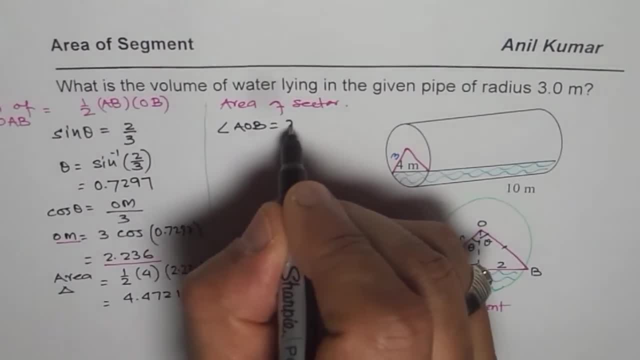 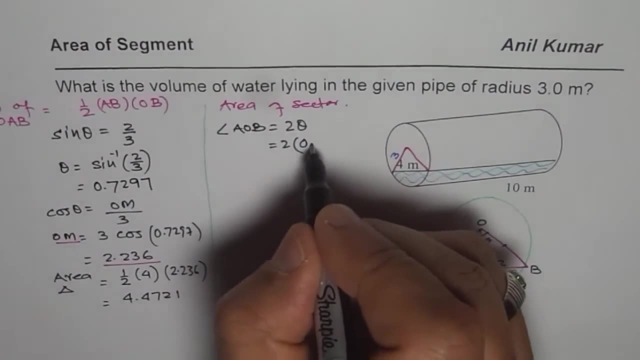 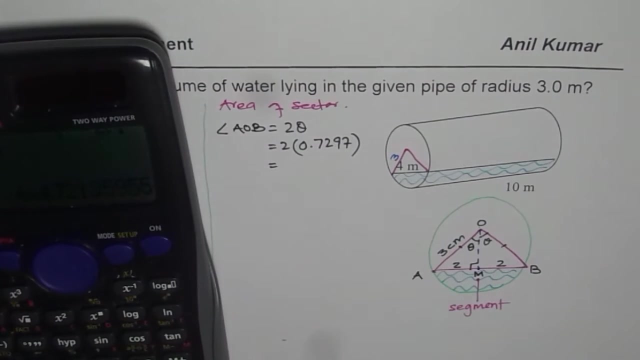 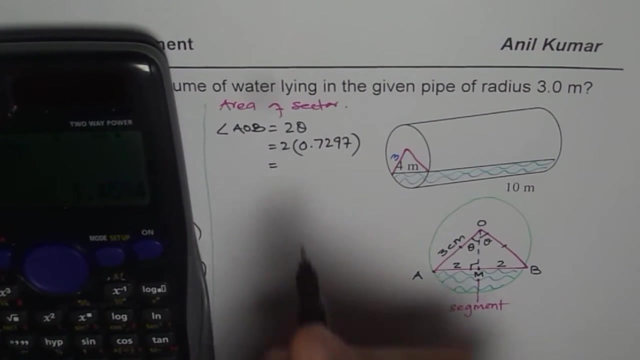 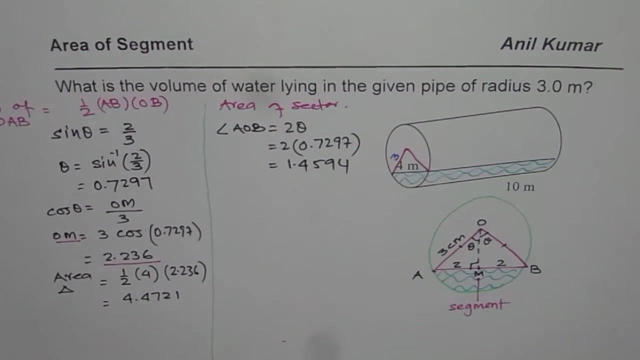 aob will be two times theta, right, theta and theta, so that is two times. we just found 0.7297 right in radians, correct? so all these calculations are in radians. we'll do two times 0.7297 equals to this is in 1.4594. use four decimal places right, that'll be good for you. 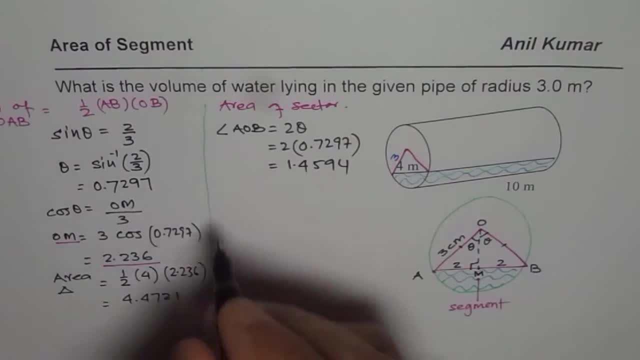 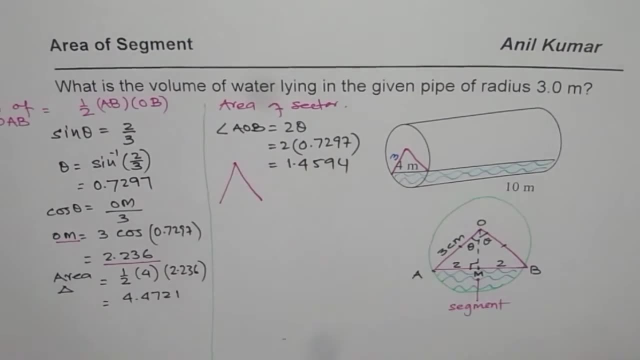 okay, so we know the angle. so area of the sector is. so now we are saying area of the sector, that means kind of like this. so let me just sketch it: be good, right? so it's kind of kind of like this. that is what we're trying to. 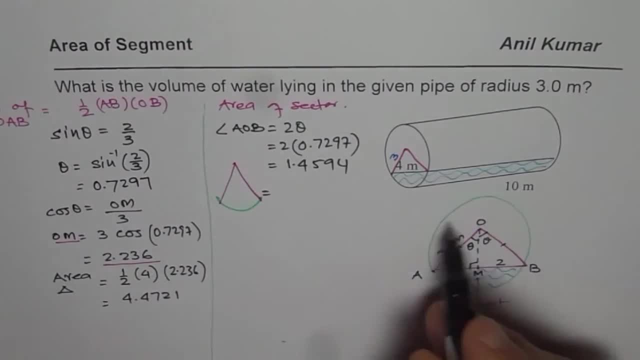 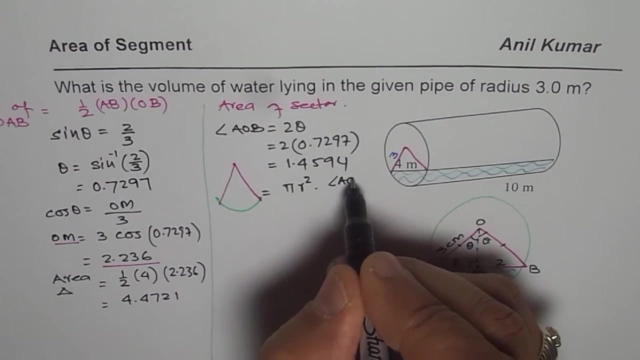 figure out is equal to total area, which is pi r square. let me write formula first times, in our case angle theta divided by two pi. so our angle is theta plus theta, two theta. let me write angle aob, right, that is better divided by total angle: two pi, perfect. so in. 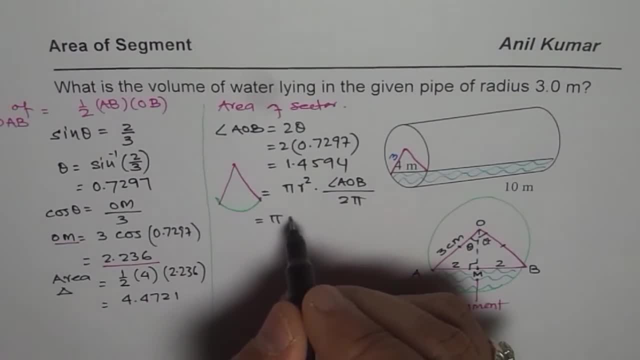 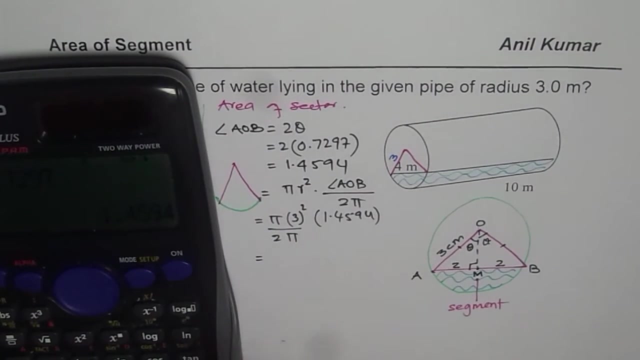 this case we are given radius as three. okay, so three square angle given to us is one point four, five, nine four divided by two pi. okay, so let's calculate. we already have one point four, five, nine four in the calculator. we'll multiply that by three square, which is nine. 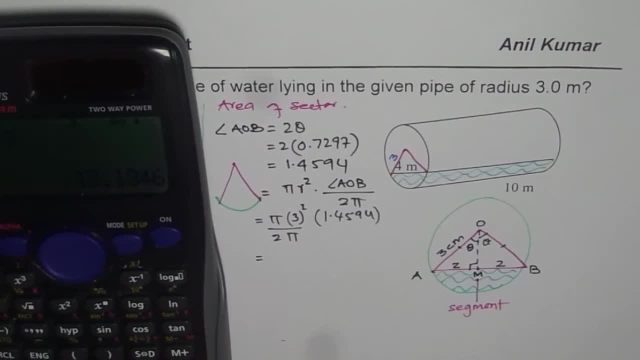 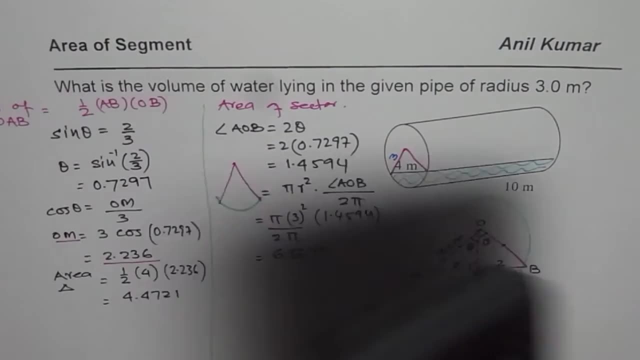 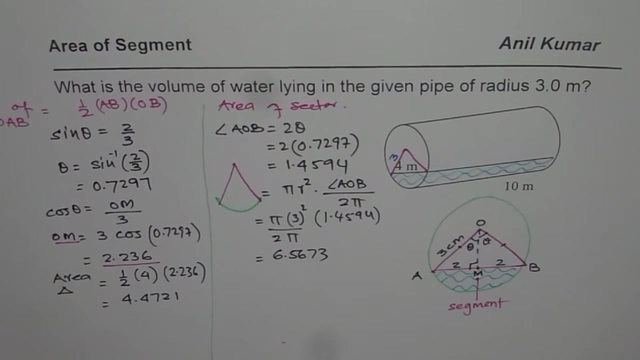 and pi, and pi cancels will divide this. Decillon ri is equal to three square divided by total two. so we get six point five, six, seven, three, as the area of sector. well, my calculations could be wrong at times, so, but at least the method is correct. I'm sure about it. good, so what you do is you? 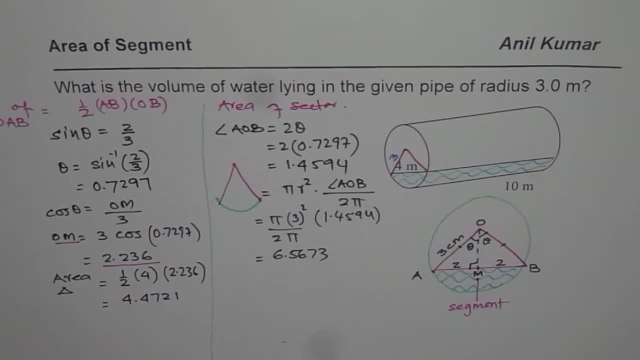 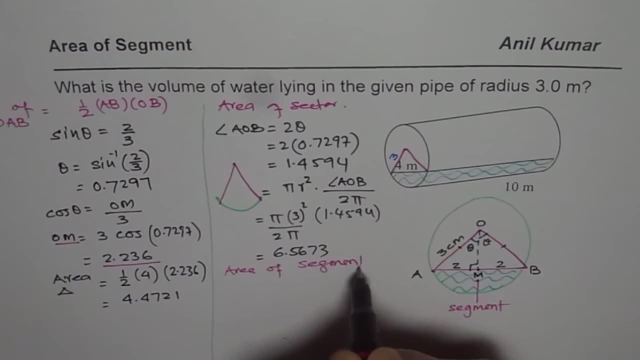 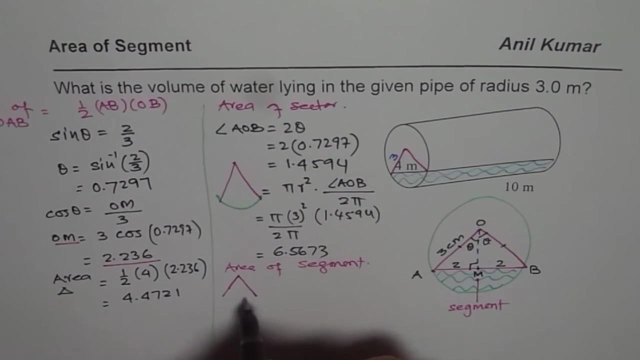 do your calculations. you once again right. okay, so now let's find area of segment, and so area of segment, which would be how, How much? Which should be area of sector? Okay, Okay, We'll do this. Okay, We have this color here. 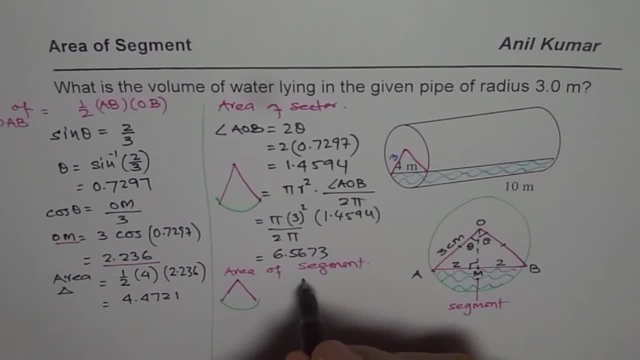 and take away the triangle itself. Okay, To get the answer. Fine, So we'll take away this from this. Okay, So we are taking away from 6.5673, the value of the triangle area, which is 4.4721.. 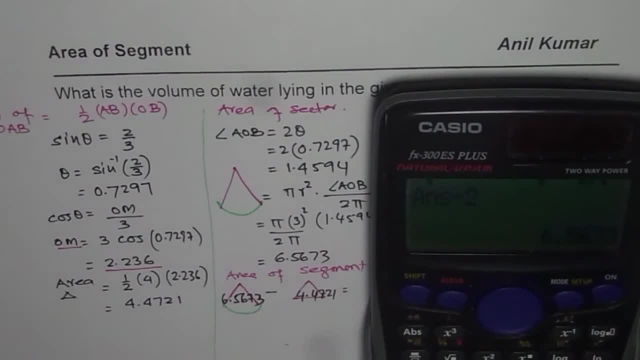 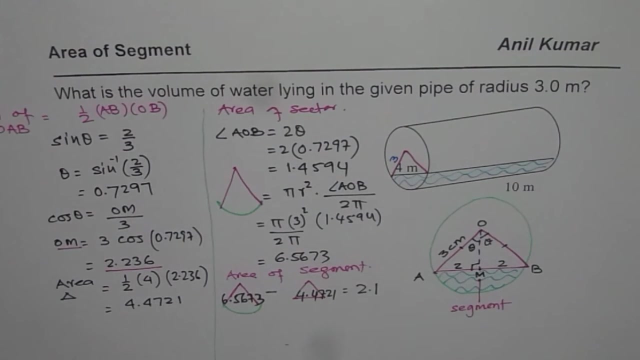 And that is equal to how much? Okay, One value is there. Minus 4.4721 equals to, in decimals, 2.09.. So let's say 2.1.. Okay, That's good. So we get area of the segment. 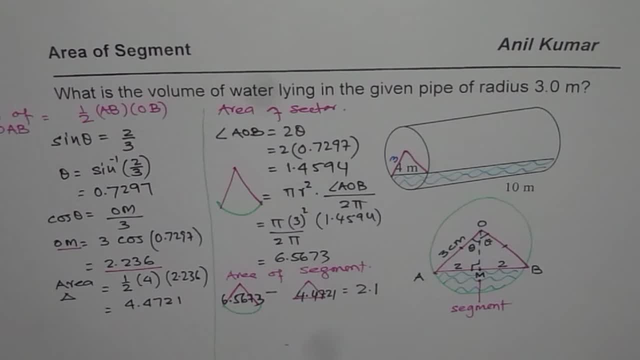 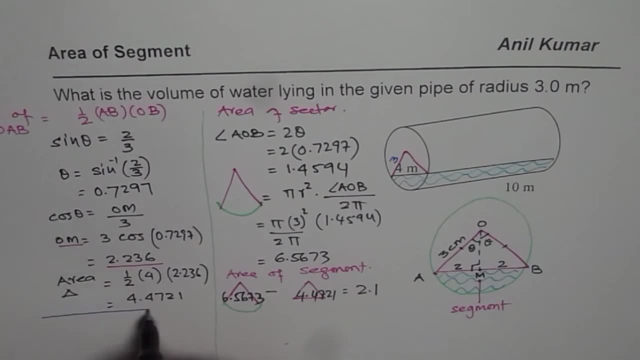 as 2.1. Perfect, And the length is 10 meters. So volume of water, let me now write down here. That's good job. So we've done the area part first, right, which we wanted to find. And now we say volume of water, right, It is how much, It is area times, length, right. 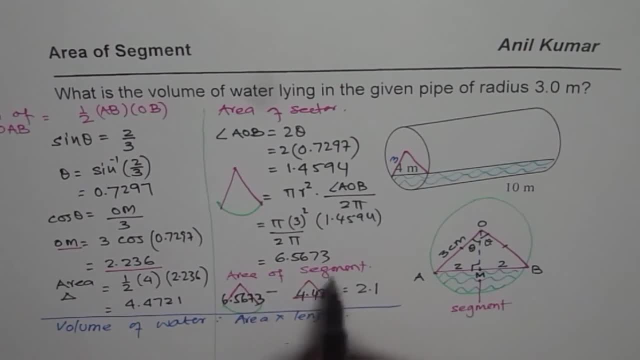 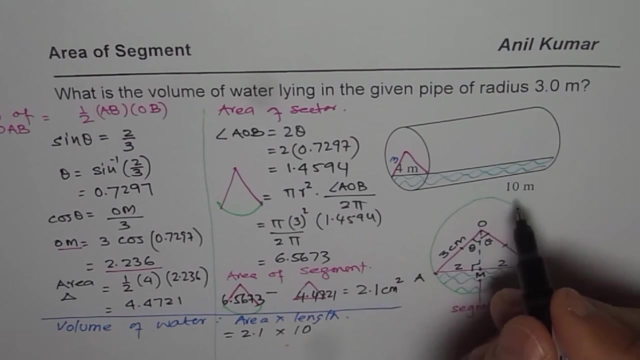 That's the formula. So in this formula, we found that the area of segment is 2.1, and we'll multiply by 10.. Okay, Now there is a mistake, Mistake. I mean this area is in centimeters square. Okay, Remember that. So this is 10 meters, right? 10 meters? Oh, no, no, Okay. 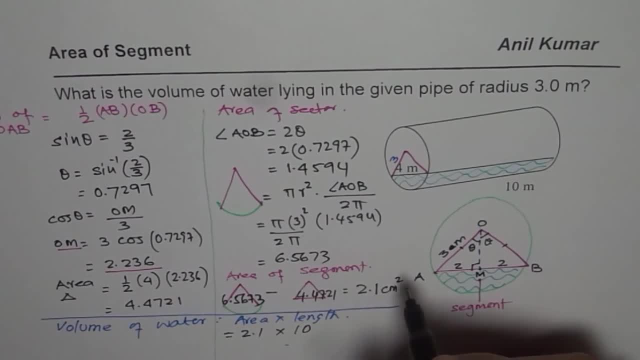 This is also in meters. I'm wrong, So this was meters. Good for us, So it is Okay. Good So we are saved. Well, at times you have to take care of the units. In this case, both are meters.